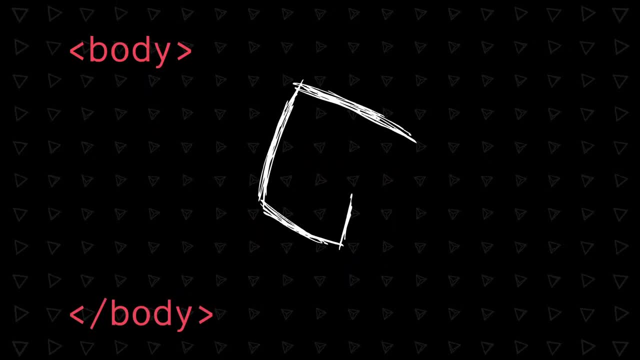 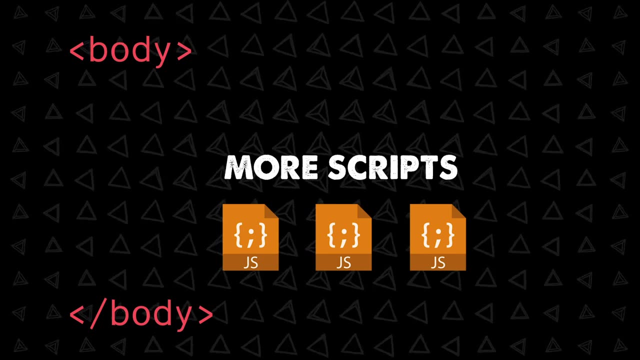 The body is everything else. It's what we want to appear literally on the page, so all of our content and main elements will go inside. We'll often add scripts to the end of our body too. This body, head and meta stuff is usually called boilerplate. It's mostly the same every time, so you 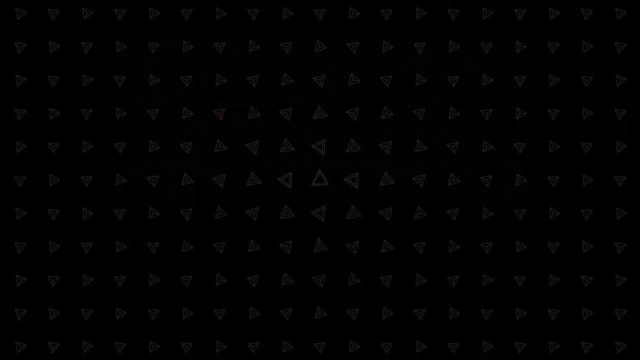 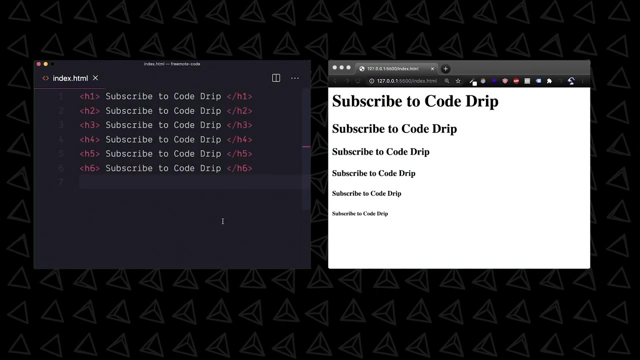 can just generate it with autocomplete in most code editors. In mine vs code you just press exclamation mark and tab Boom. Now let's talk about the most common HTML elements. You have these titles, but you can also have paragraph elements which you can use to separate long form. 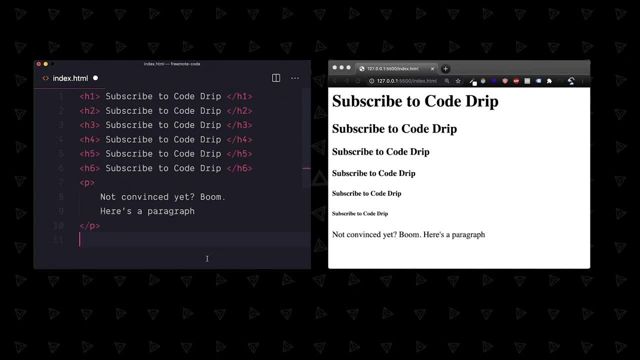 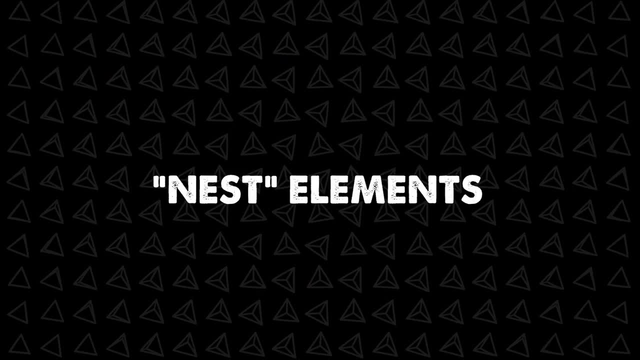 text content. There are more text elements, too, that modify your existing text, like underlining, making it bold, italic, but these are a bit weird because you can also use CSS to do this. Did I mention, by the way, you can nest elements inside each other? I think I did, but you definitely can. 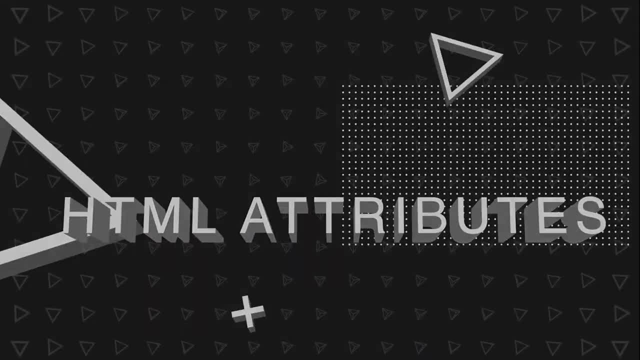 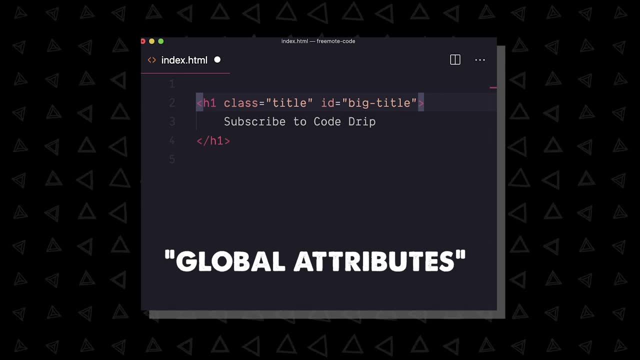 Now let's talk attributes, which can modify your elements or add properties to them. Attributes go inside the opening tag. There are global attributes like classes and IDs that you can add to any tag out there. A class lets us style an element or select it with JavaScript later on, when we add CSS and 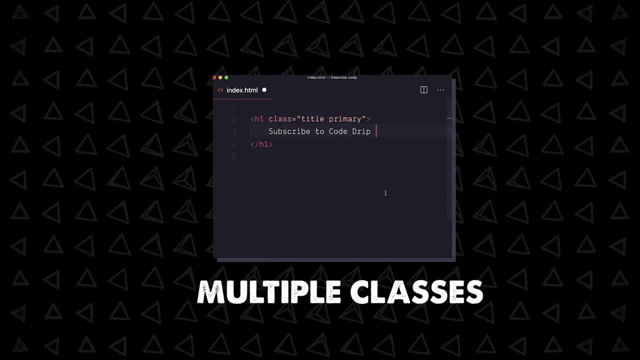 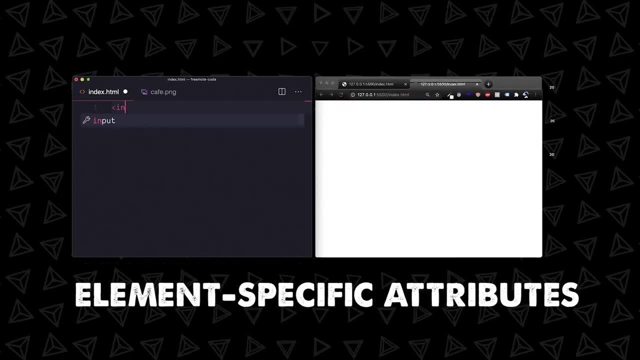 JavaScript Pretty useful. We can apply multiple classes with a space and reapply the same class to any element. Other attributes are element specific. For example, if we want to load an image, we would use an image tag, and the image tag requires a. 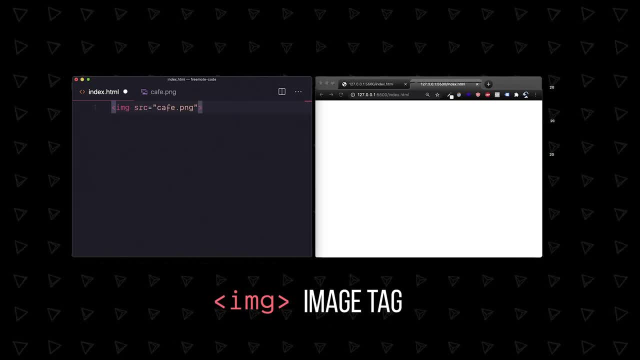 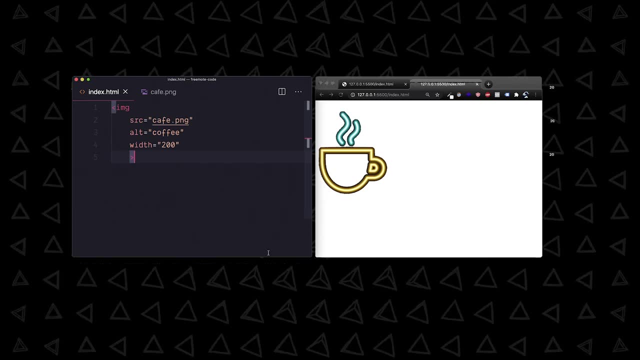 source attribute. to work, The source should be the URL of your image. Then it works. Images have a lot of optional attributes too: Alt for backup text width and height. Let's keep going. Anchor tags are links. They're super important for navigation and require an href attribute. 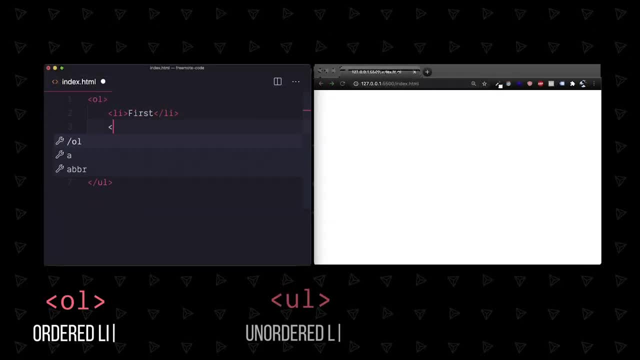 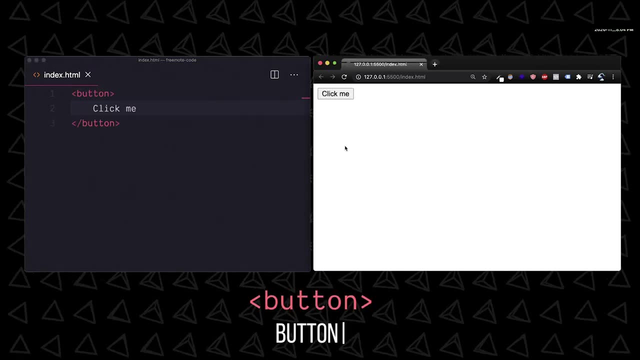 that is the URL you want to link to. We have ordered and unordered lists depending on whether you want numbers or bullet points. Use the li tag inside them for each item. You can create button elements and use them as links, or style them with CSS and add JavaScript. 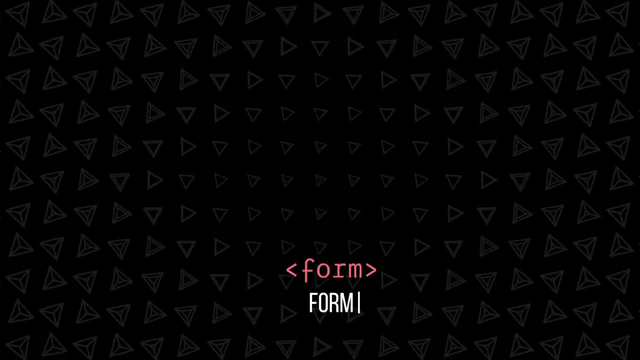 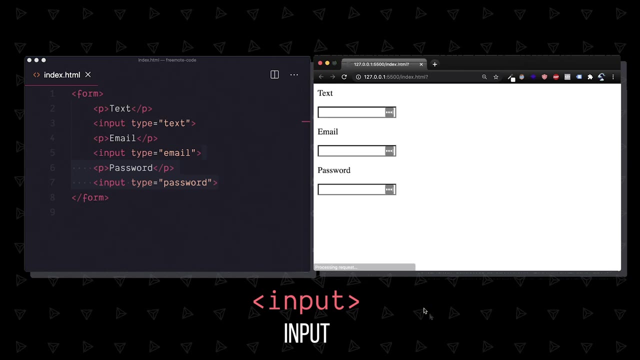 to do some pretty cool stuff. Next up, we've got forms. With these, users can log in, create posts, make payments and more, And you'll do this by wrapping one or more input elements. Now you can have the basic text, but you can also have emails and passwords Beyond that. 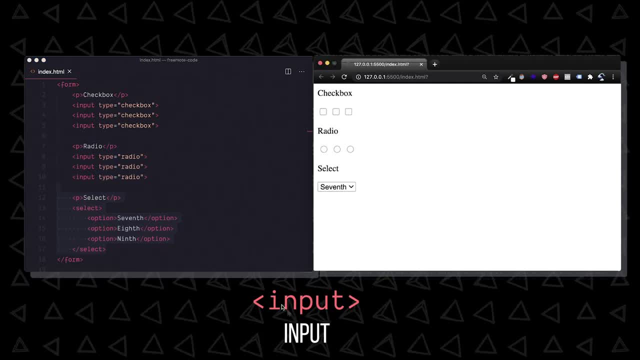 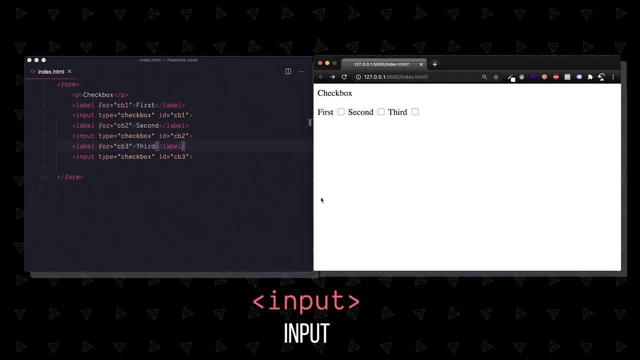 you can have checkboxes, radios and select dropdowns. You can link an input to a label with an ID on the input and a for attribute on the label, And when you click the label it will activate your input. I'm using checkbox as an example, but this works for all the inputs. 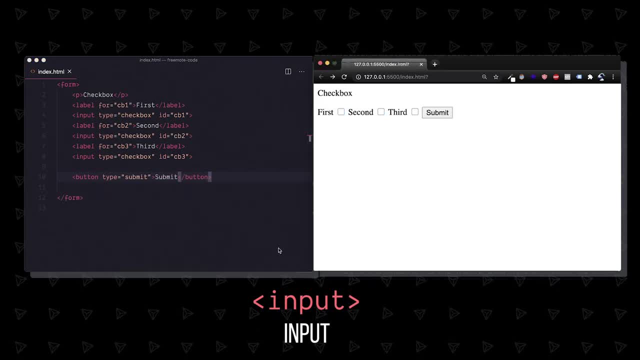 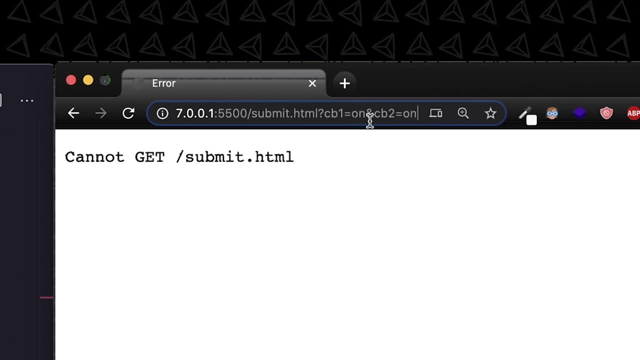 The submit action can be triggered by a button or, in certain cases, by hitting enter For form submission. add the action attribute and then the name attributes to your individual inputs, which will put their values in the URL when you submit. And there's a bunch more. 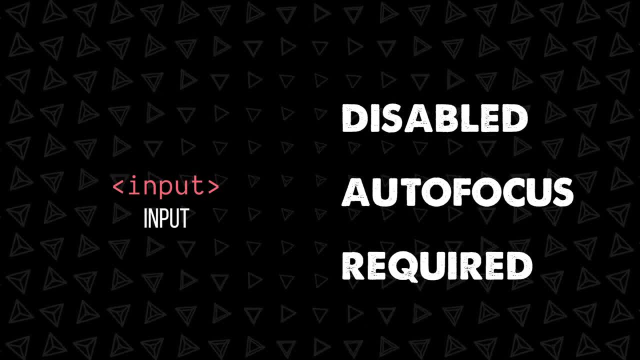 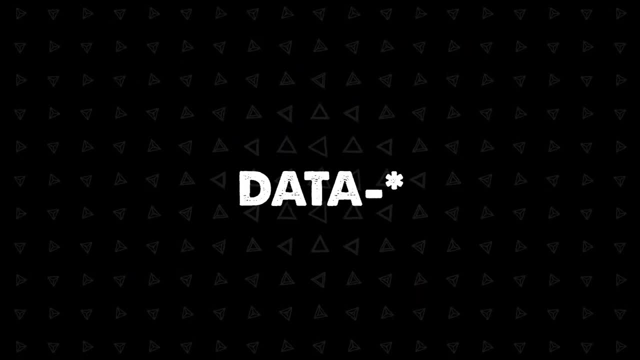 attributes for inputs like disabled, autofocus and required. Most people still pull up a reference for this, even if they've done it a hundred times. There's one more weird attribute. you can put on anything too: a data attribute. You can store any string data on an element. 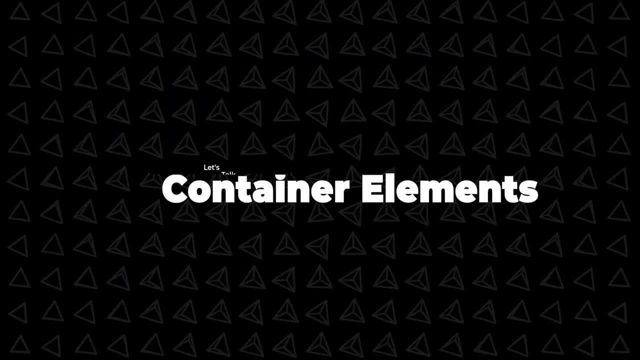 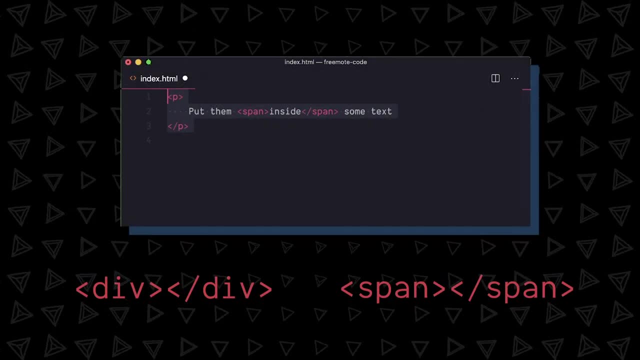 and then retrieve it later. Okay, let's talk about container elements. You can put stuff inside a div or a span and then style or select this container. Spans are for inline text and divs are for sections, but an anti-div movement has actually emerged. 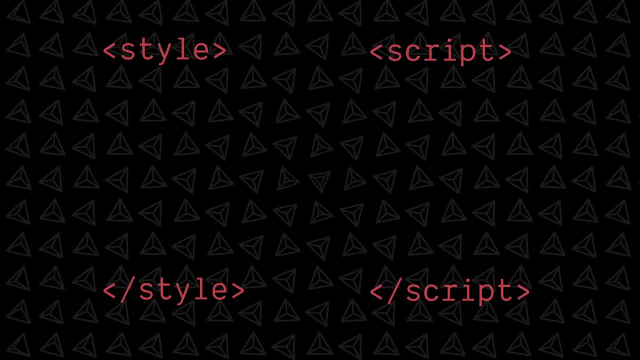 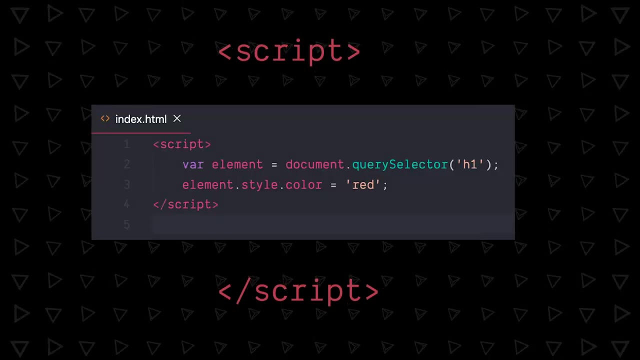 More on that soon. Last up, we've got style and script tags, which flips the language you're writing between the tags Inside: style, CSS and script. you guessed it? JavaScript. So you can write all three languages in a single HTML file. but to keep things organized you should generally separate them. Just make a single HTML file and you're good to go. So let's take a look at some of the things that you can do to keep things organized. You should generally separate them. Just make a style, CSS and a script- you guessed it? JavaScript- So you can write all three languages in a 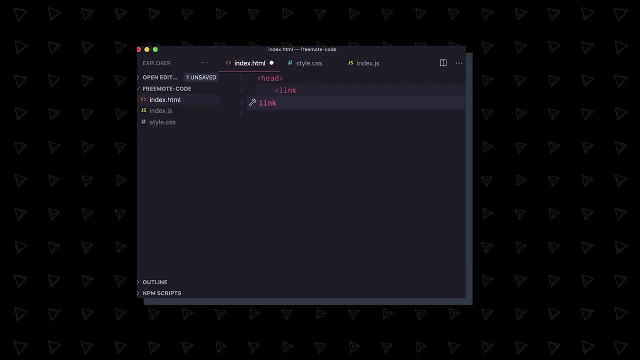 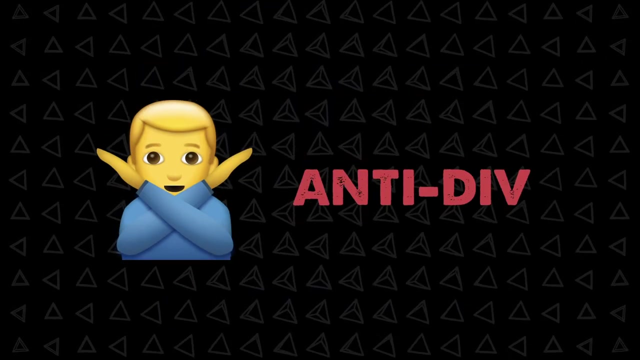 single HTML file, but to keep things organized you should generally separate them. Just make a second file, it's not hard, and then you can import that file like so for CSS and like so for JavaScript. Finally, let's talk about that anti-div movement called semantic HTML Instead. 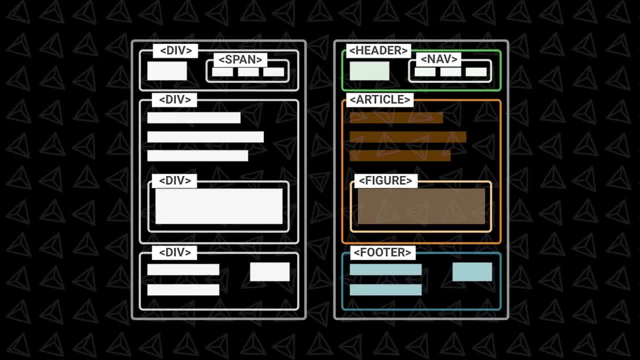 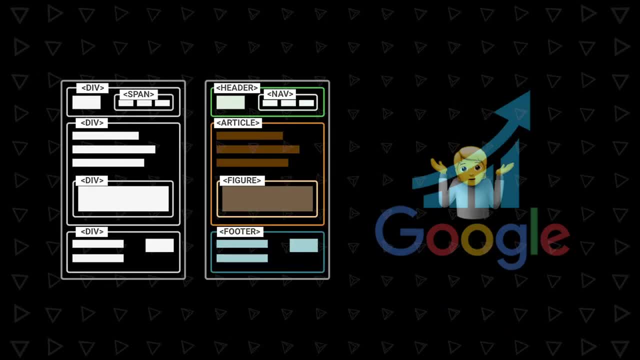 of a div, which is a generic container. you're supposed to use more descriptive containers like these. These containers don't function any differently, but they're supposed to be better for search engines and for developers, assuming you name your containers correctly, that is. 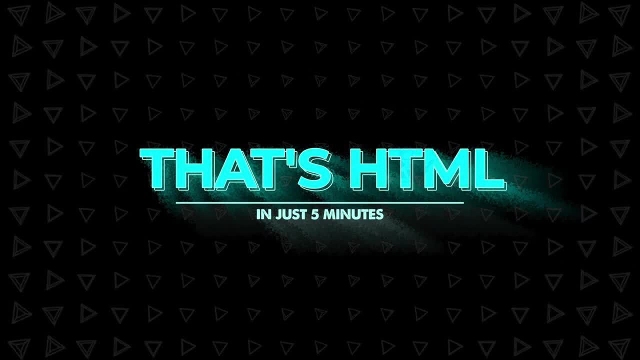 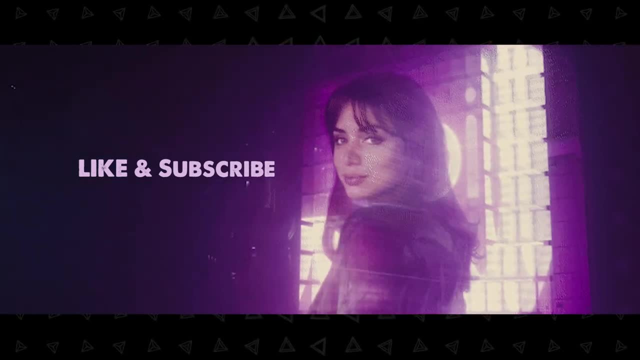 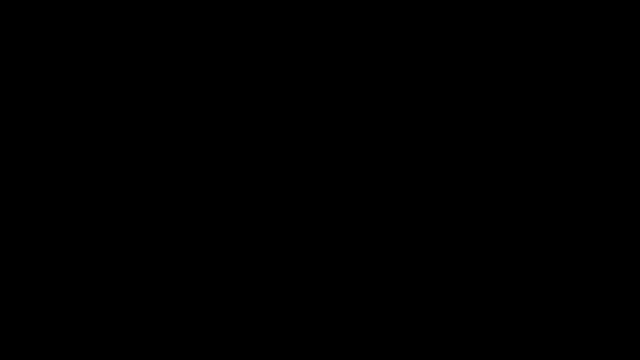 Anyway, that's HTML in five minutes. It's really not too bad or complicated. Hope you learned something. Let me know what you want me to explain or build in five minutes and I'll see you real soon.